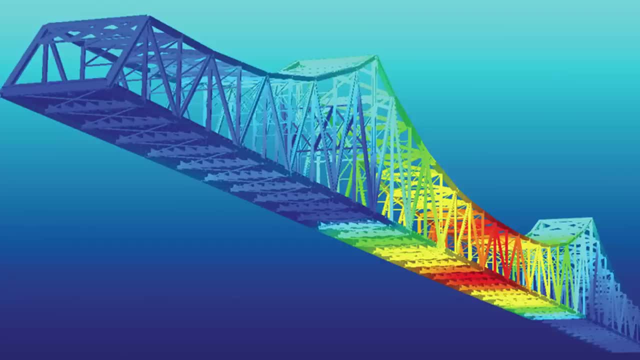 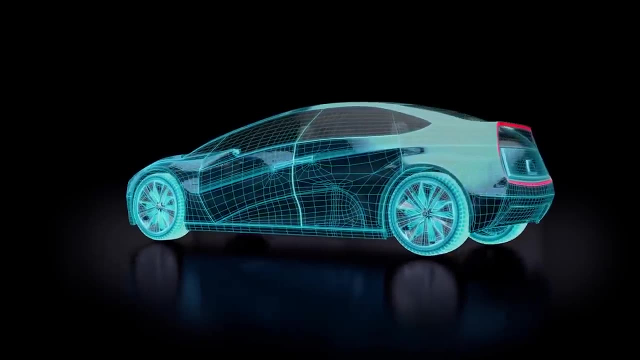 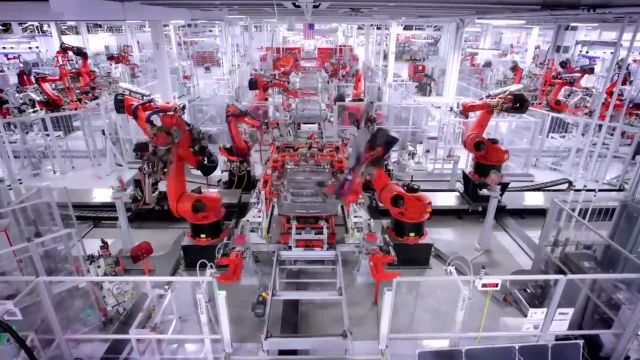 to often differential equations in the background, And you know we don't need to know exactly how a car will deform in a crash, for example. We need accurate solutions that allow us to maximize safety, minimize any prototypes that might need to be made, and so on. 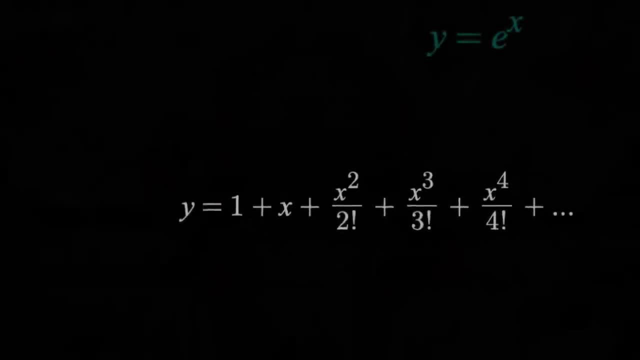 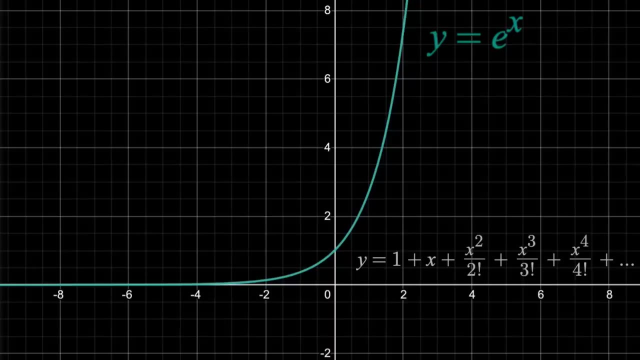 Now, as a real quick overview, here we have the Maclaurin series for e to the x. Simply put, this is a polynomial that approximates e to the x better and better the more terms you include. If I just graphed, y equals these first two terms. 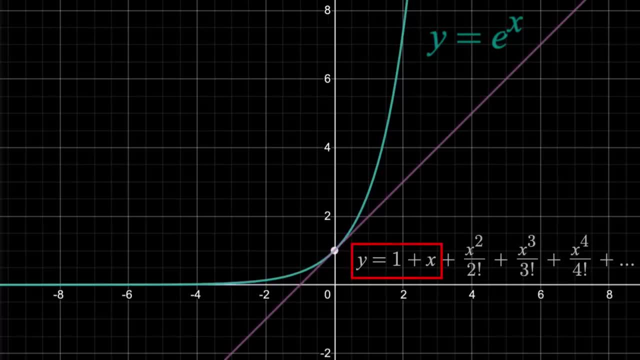 Then we get a tangent line approximation, which is only a good approximation for x values close to zero. But the important thing to note is that this function and e to the x have the same first derivative and y value at x equals zero. If I go out to a third term, we get a parabola. that is an even better approximation to e. 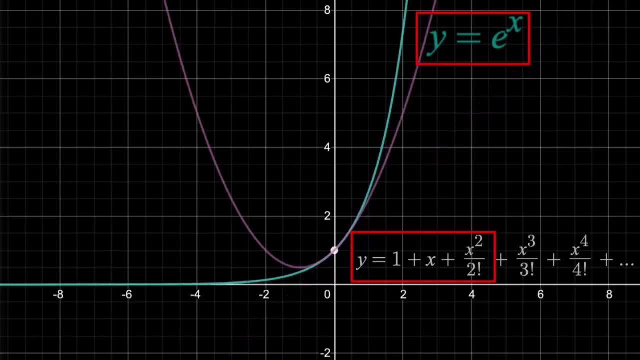 to the x around zero And this function and e to the x have the same first and second derivative, just at x equals zero. If I go to four terms, the approximation gets even better. And as we keep going including more and more terms, the approximation keeps improving. 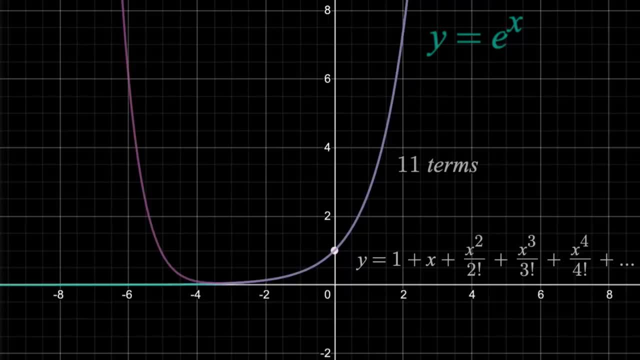 Although I'll stop at 11 terms. if I were to go on forever, we would get a perfect approximation and the curves would look the exact same. The general equation for the series looks like this, And all this is is a polynomial whose derivatives at some- x equals a- will match those of your. 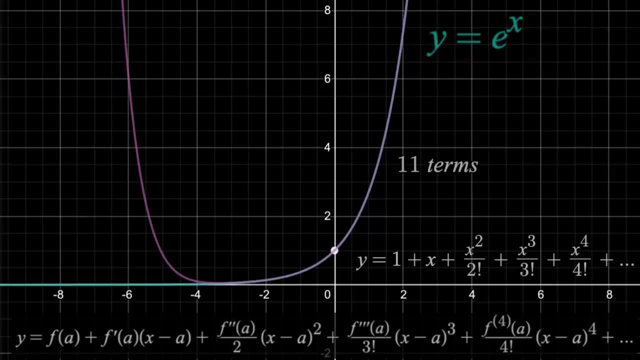 original f of x. When a is zero- Which means you're right- The approximation is centered around that x value. like we see here, We have a Maclaurin series. When we move that center point to anywhere else, then this is called a Taylor series. 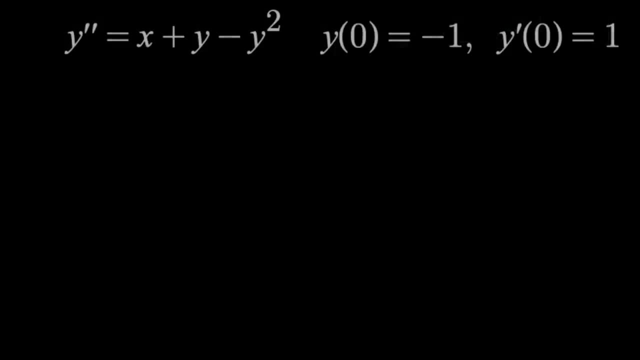 For our first actual example, we're going to pretend this random differential equation with initial conditions that I just got from my textbook yields a solution that's very important to an engineer or scientist. The problem is that this is a non-linear equation and those are normally difficult or impossible. 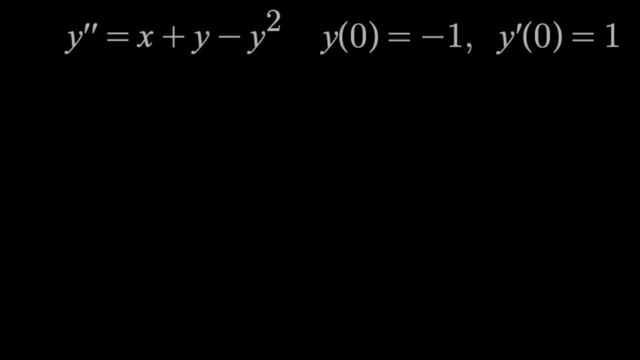 to solve. But we can get an approximate solution Because, remember, we can represent equations sometimes perfectly just through a polynomial And if we know the derivatives and y value at some point, like x equals zero, then we have everything we need to find that equation. 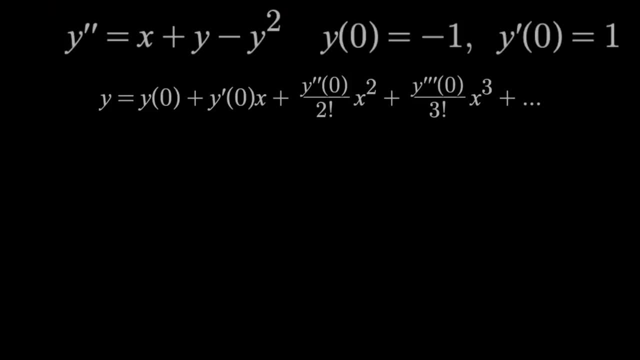 Since this y equation is going to represent the solution to our differential equation, we already know the first two coefficients, because that's what the initial conditions are: y of zero and y prime of zero. so we can already get started and plug those in. 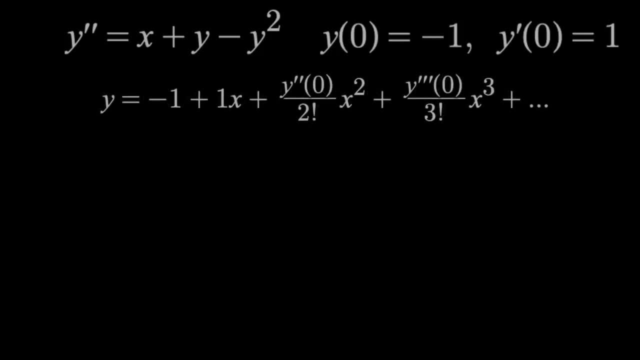 Those were kind of freebies, but the other coefficients aren't hard to get. For y double prime of zero, all I'm going to do is plug zero into the original equation. What you see here is just the same equation, except anywhere there's a y or y prime, or 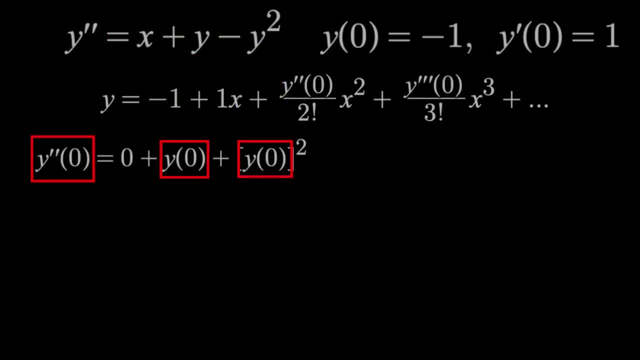 whatever I include it in- of zero, and then also zero went in for x. We know y of zero from that initial condition though, so if we plug that in, we get y. double prime of zero is negative two, And we have another coefficient of zero. 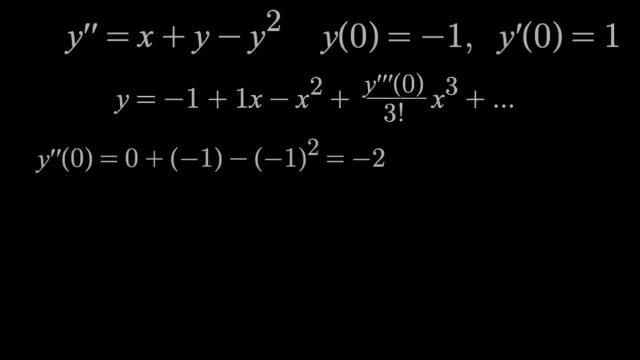 We plug that in, We get the same coefficient in our polynomial. For the fourth term we have to take the derivative of both sides of the original equation, which yields y triple prime of x equals this. So to get y triple prime of zero, I'll do the same thing as before, writing the same. 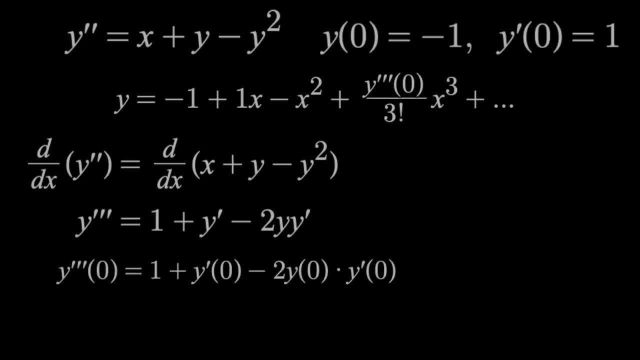 equation with y and y prime of zero, And then again, these are all just initial conditions which we can plug in to see that the output is four. If we did this forever, we would get an entire Taylor series. that is the solution to the. 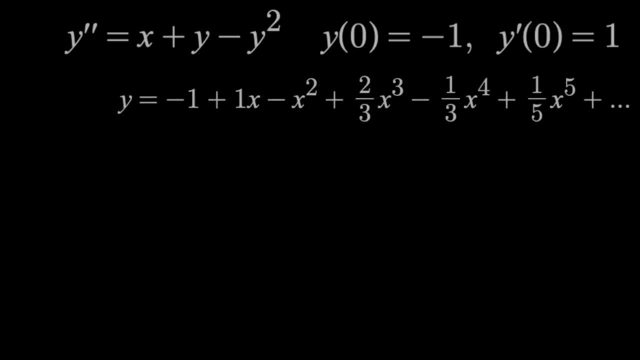 original differential equation. Now, this doesn't mean there's an infinite radius of convergence and we have a perfect approximation for all values of x. But if we have a positive radius of convergence then we can get local solutions, Like if this equation represents force versus position and we want to know the force at. 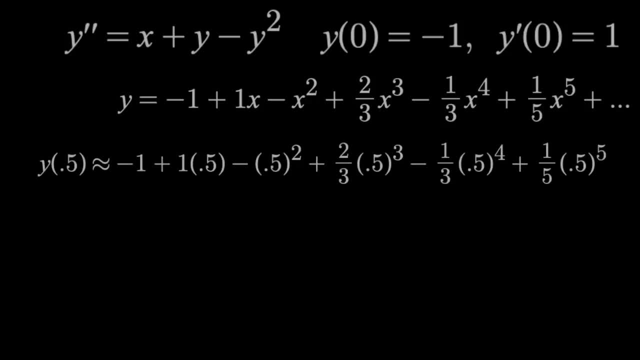 0.5 meters kind of close to zero. we could plug that into the first several terms and get an approximate output. Now the same thing happens if we plug this into the first several terms and we get an approximate output. Now the simplest kind of approximate you can do with these is some fast math. 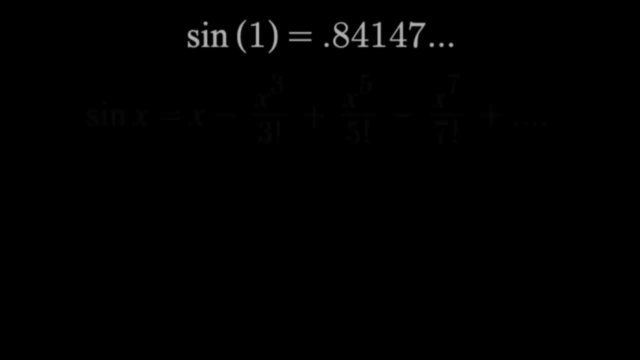 Like you would not know, this is sine of 1 without a calculator. but you could use the Maclaurin series for sine of x and plug in 1 to, let's say, the first two terms. That gives you an approximation that's fairly accurate. 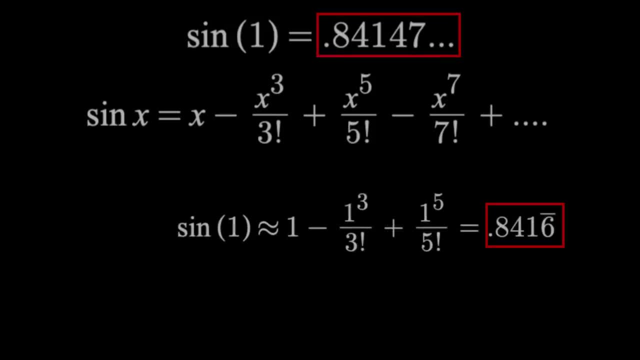 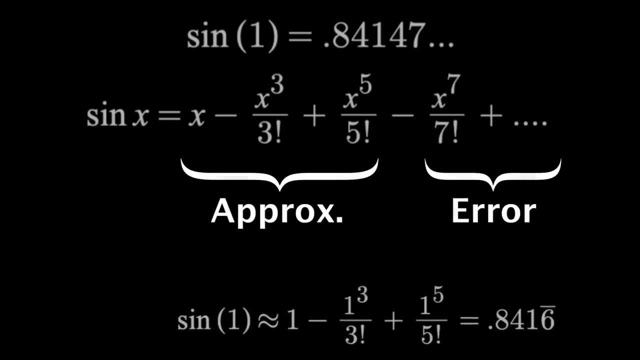 Go out to a third term and you get something even closer. However many terms you include is your approximation and what's left is your error. in this case, it's what you're leaving out of what would be a perfect approximation. but since the 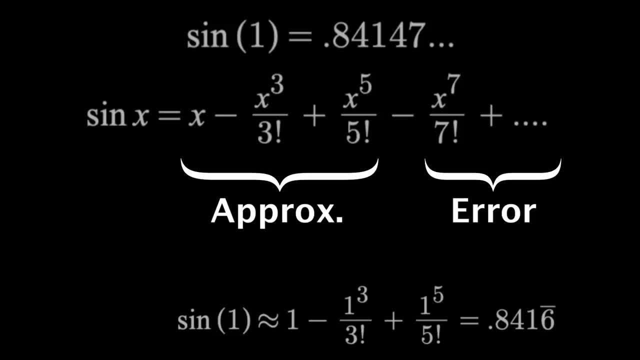 denominator gets so large, then that error is fairly small. And if x is close to zero, then we could approximate with only one term and the error itself would still be pretty minimal. So we can say: sine of x or sine theta is roughly equal to theta for small input angles. 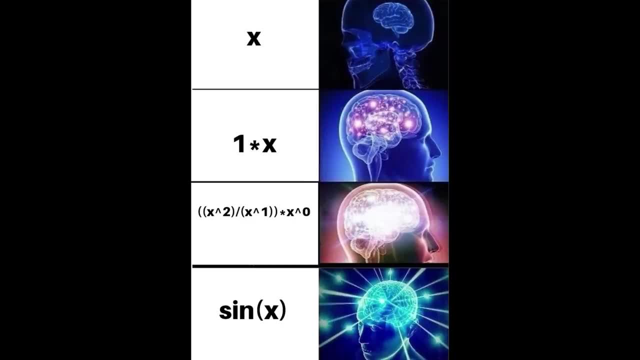 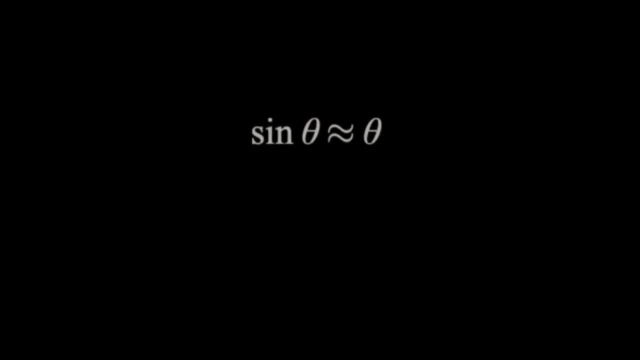 and unless this is your first time on the internet, you've probably seen this memed many, many, many, many, many times, But it does simplify things. The classic example is in regards to a simple pendulum. The equation that represents its motion is difficult to solve, but for small values of 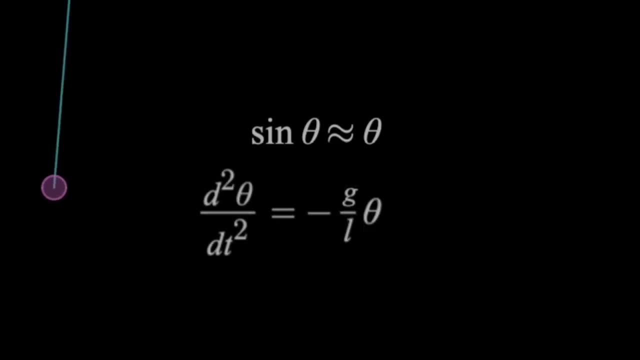 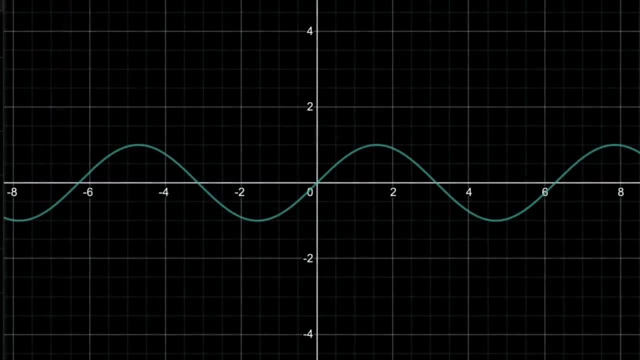 theta. we can approximate sine theta as just theta, making the equation much easier to solve Graphically. we're saying that sine of theta or sine of x is roughly the same as y equals x, which only works for those small angles close to zero. 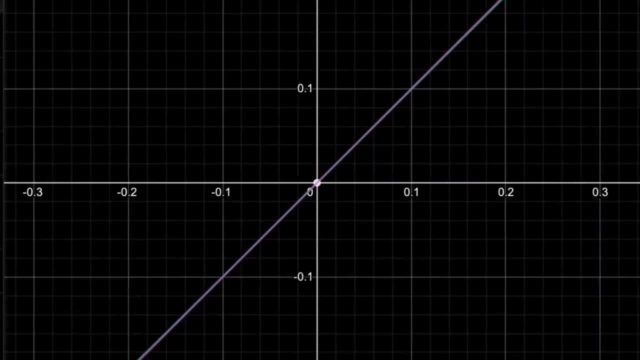 That's why we can do the substitution with that small angle assumption. In fact, if we allow theta to reach a maximum of 10 degrees, you'll find the percent error between the tangent line and actual sine curve changes from 0.5% to 0% and back. 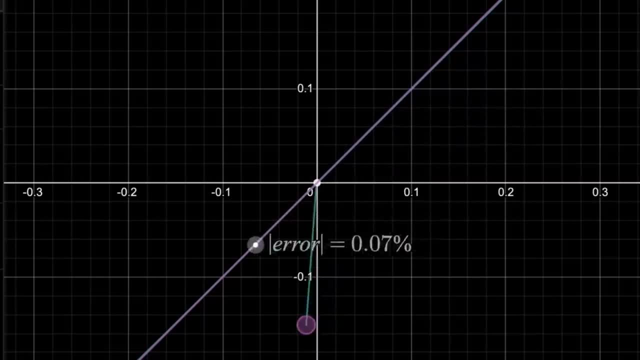 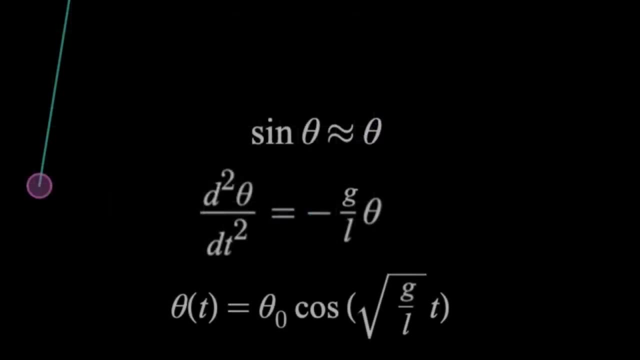 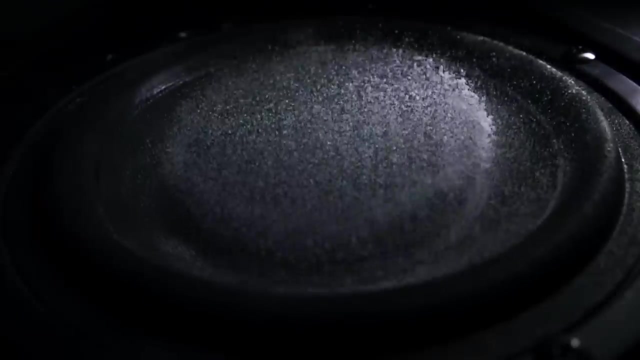 Pretty good, So we sacrifice a little accuracy in order to get a much easier equation to work with. that has a fairly simple solution. Taylor series also show up outside of differential equations, though If you've taken a first year physics course, you may have learned that the speed of sound 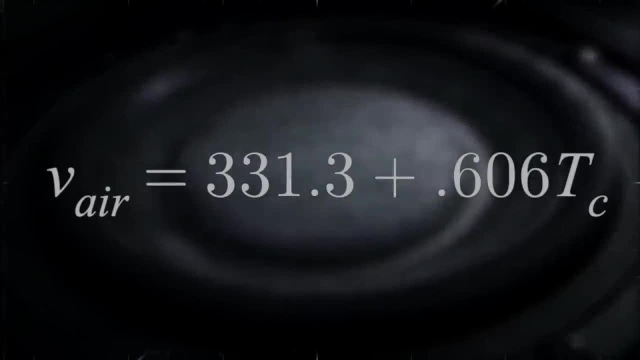 in air is determined by this equation here, where t is the temperature in celsius. So if you've taken a first year physics course, you may have learned that the speed of sound in air is determined by this equation here, where t is the temperature in celsius. 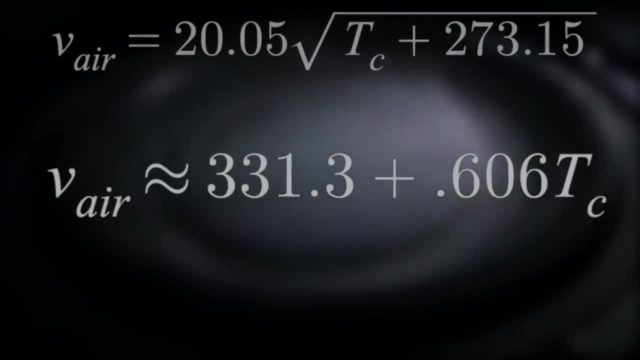 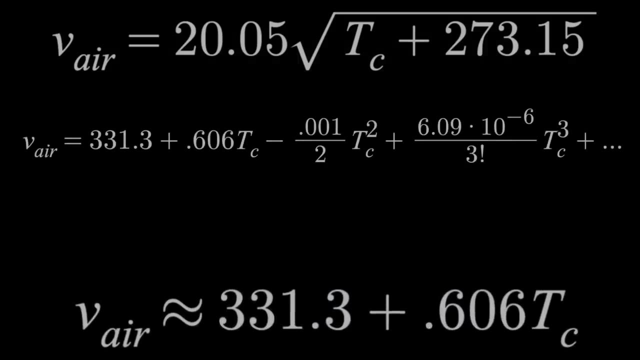 This is only an approximation, though that comes from this equation. So how do we get the approximation? Well, we find the McLaurin series for the more accurate equation up top and then just use the first two terms. So yes, another tangent line approximation that will work around. t equals zero. 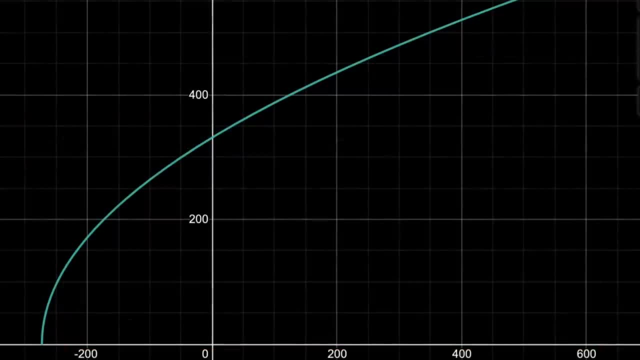 Graphically you'll find the percent error between the actual velocity equation and the linear approximation only reaches about 0.5% once you get to roughly 60 degrees celsius. So for typical everyday temperatures you'll find that the percentage error between the 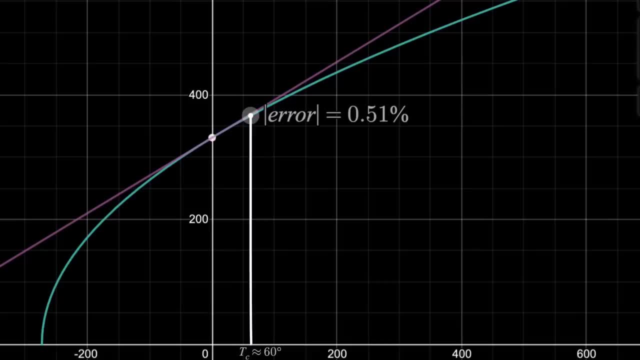 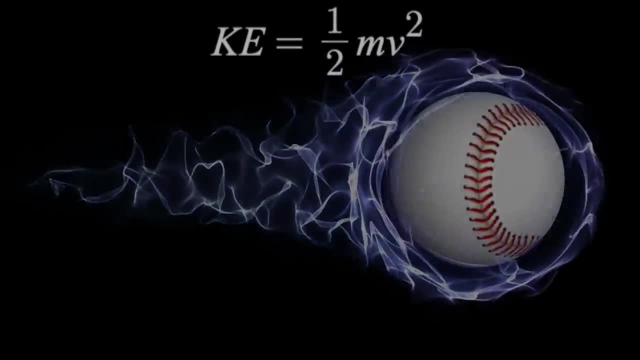 actual velocity equation and the linear approximation only reaches about 0.5% once you get to roughly 60 degrees celsius. But yeah, even in case of temperatures the approximation is pretty accurate. Or in basic physics we learn that kinetic energy is found by ½mv squared, but later. 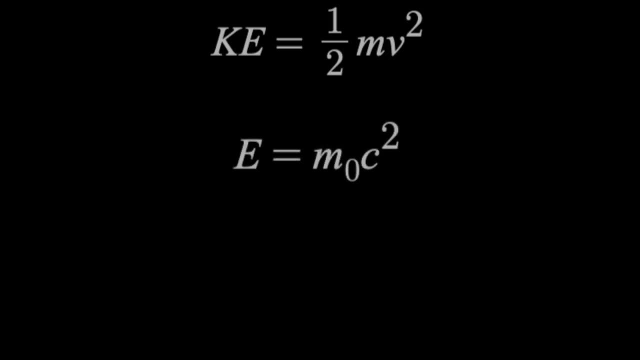 on, you learn that objects, even at rest, have intrinsic energy determined by m0 c squared, And m0 just refers to mass when the object is not moving. Anyways, adding this with the ½mv squared gives us sort of the real total energy. but 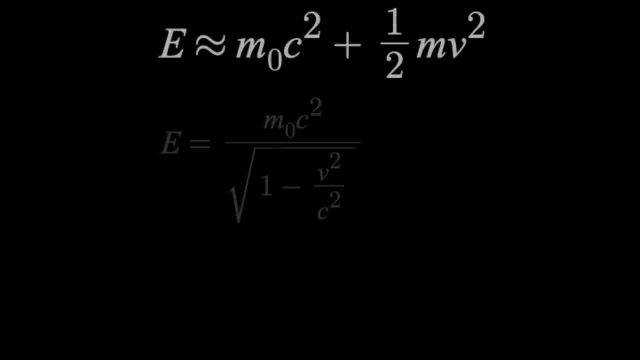 turns out, this is still only an approximation for energy. that includes MC squared, but also velocity. You'll notice, if V is zero, the energy is just M naught C squared, as expected. Now if we expand this into a Maclaurin series treating V over C as a single variable, then we get this here At: 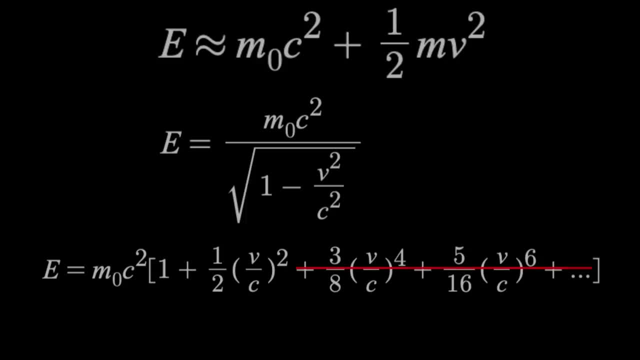 low speeds. we can ignore all of these terms because the speed of light C is so much larger than V and after distributing the M naught C squared, we get this here: our low speed energy approximation. So these Taylor and Maclaurin series can help us see some approximations that aren't obvious from the original. 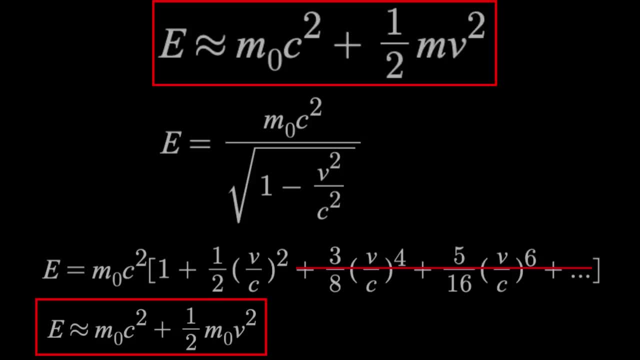 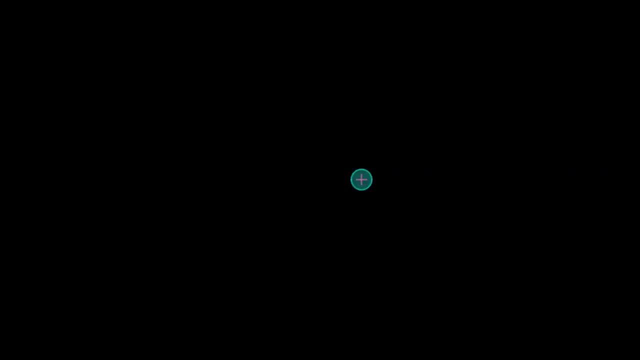 equation In this example I had never done in school, but it has to do with asymptotic behavior. If we have a single positive charge in space, then the electric field at some point is inversely proportional to the distance from that charge, squared Meaning if the field strength here is some E naught. 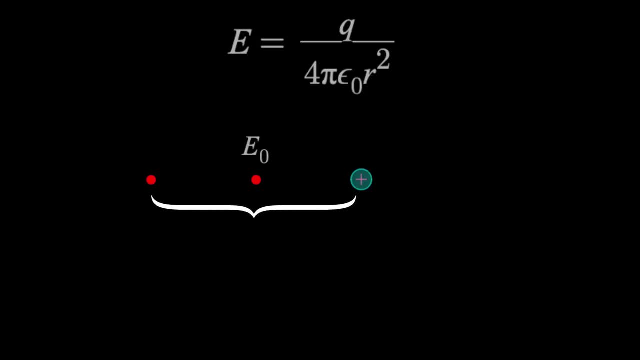 then at a point twice as far away from the charge as the field strength here is, four times the field strength squared, The field strength will be four times weaker. But what if we had two charges of opposite signs sitting near each other? we'll say both a distance A away from the origin. The question is if we're far. 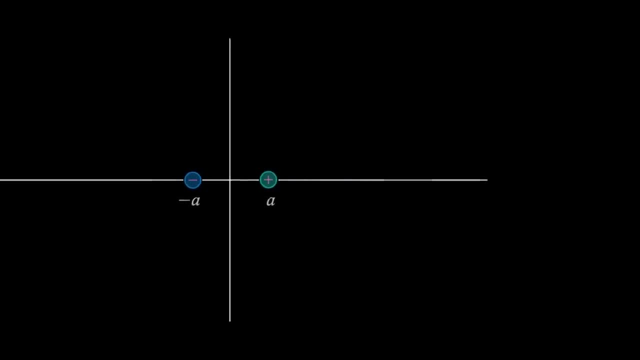 away from the origin on that same axis, what kind of behavior will we find, Like what happens to the electric field now if we double that distance from the origin? Well, the total electric field at some point on the right at a distance X from the origin, is this here, if we assume the charges have the 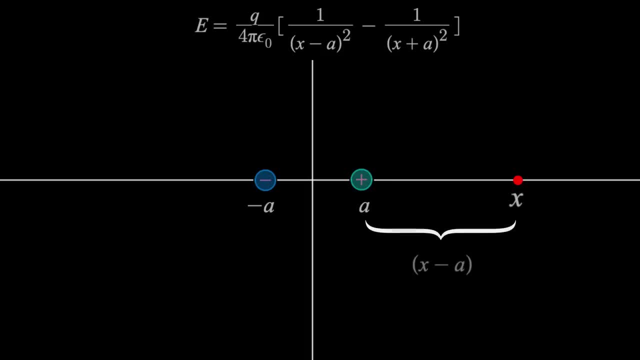 magnitude. this length here is x minus a, and this is x plus a, which is where those distances come from. what we're going to do is first pull an x squared out of the denominators and rewrite the equation as such. now we can finally apply a taylor series for these two. 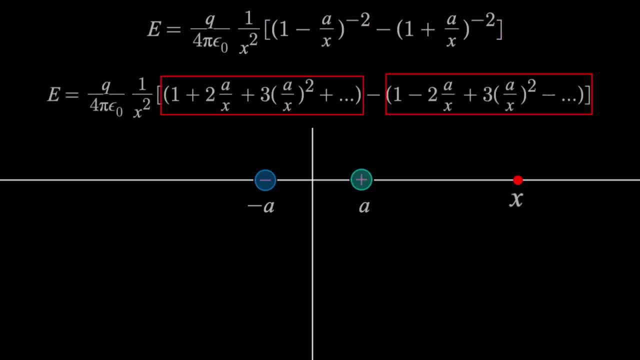 functions and those series will look the exact same, except for the alternating signs for the one on the right. so a lot will cancel here, like 1 minus 1 or 3a over x, squared minus the same thing, and so on. for every other term the rest will combine to make like 4a over x. there'll be an. 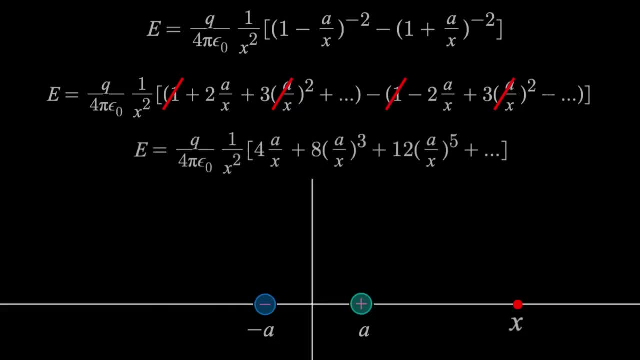 8a over x cubed and so on. but since we're saying x is much larger than a, we can ignore all these higher order terms and just keep the first. thus we can approximate the e field as shown, which is inversely proportional to the distance from the origin cubed. so to answer our earlier 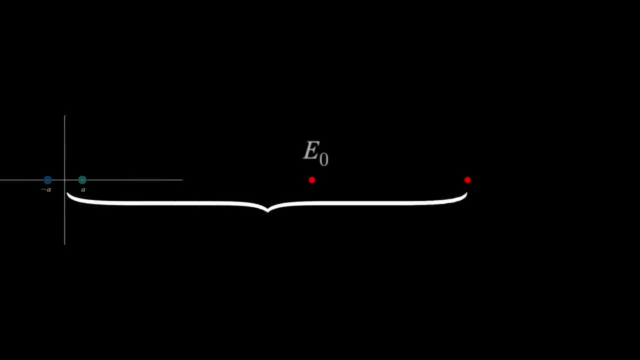 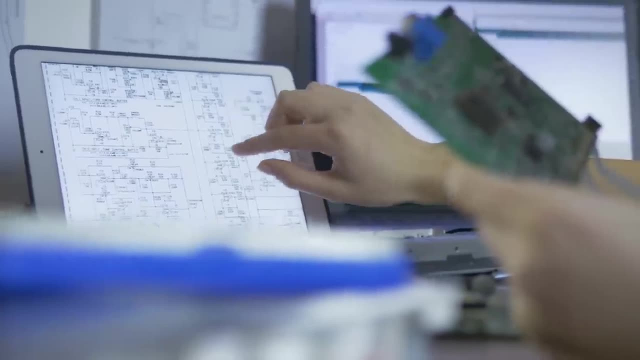 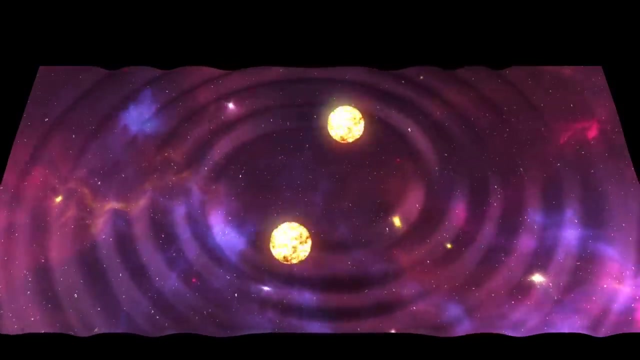 question. doubling that distance makes the field strength about eight times weaker. so i know this video has been a lot of approximating, but it's because in the real world we simply have to. i mentioned a lot of engineering examples, but especially in physics, very often approximations come down using taylor series to turn some complex function into a linear or 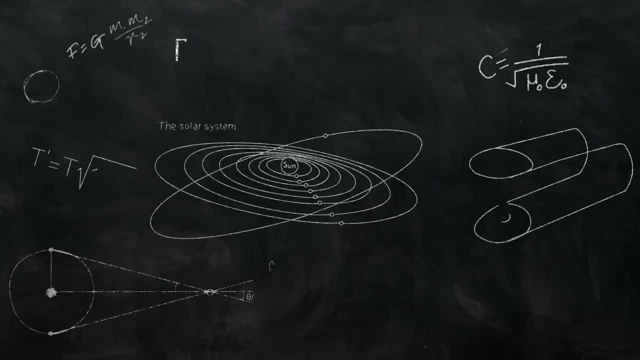 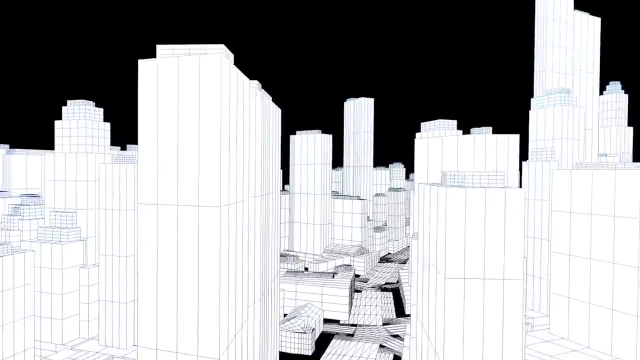 quadratic one. so although it doesn't sound pretty good, it's still a good idea to try it out. if you are a math professional, being good enough is often what we're after. there are actually entire courses dedicated to numerical or really approximation methods that i might do a separate video on, but 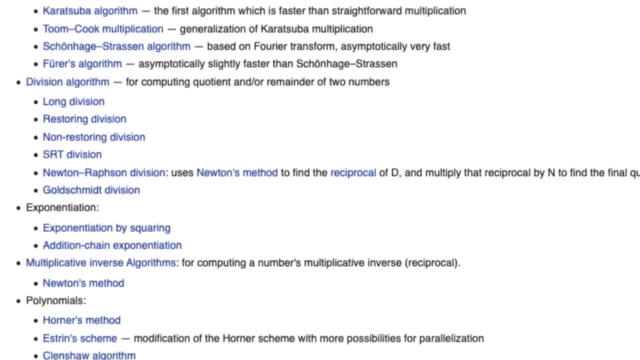 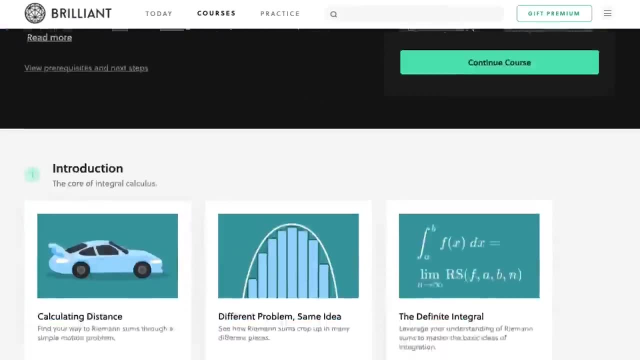 for now, we'll leave it here. if you're interested in learning more about this stuff, though, you can head over to brilliantorg, the sponsor of this video. their integral calculus series is where you'll find problems related to power series, as well as other calc topics like ratio and root. 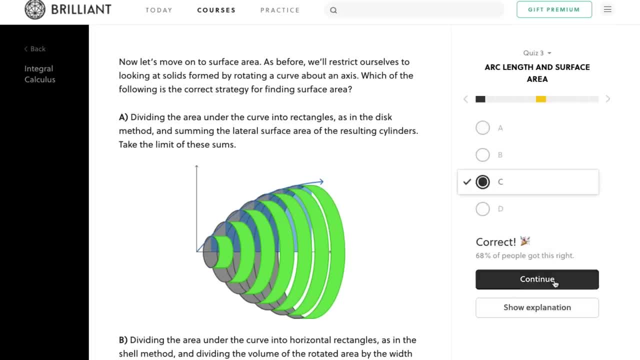 tests, arc length and surface area, integrals, various integration techniques and more. so just your array of questions real quick. but most units are not good enough for tänor. it's just time and work and more. If you're in a more advanced math class then you might enjoy their.